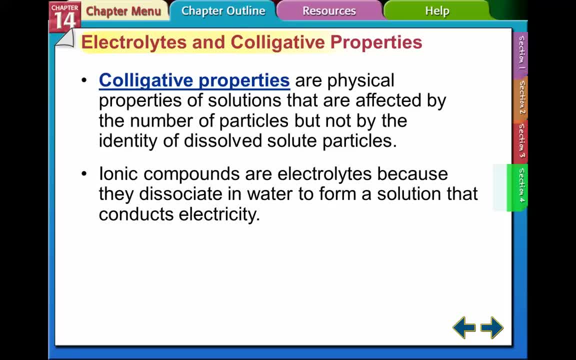 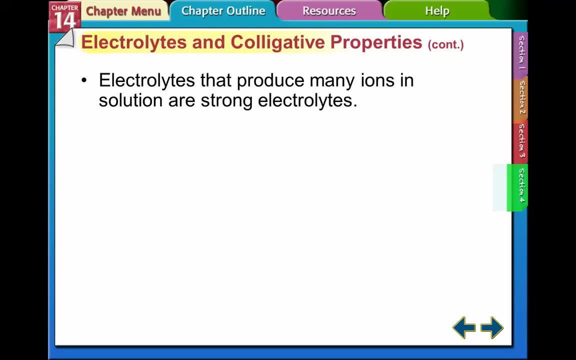 And ionic compounds create electrolytes because they disassociate in water to form a solution that can conduct electricity. So that's kind of a review. And some molecular compounds are also electrolytes because they have polar properties on them, Electrolytes that produce many ions in. 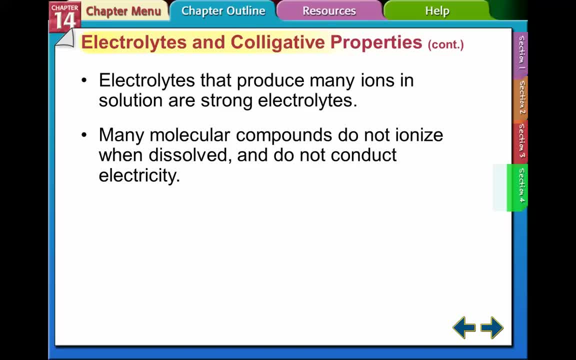 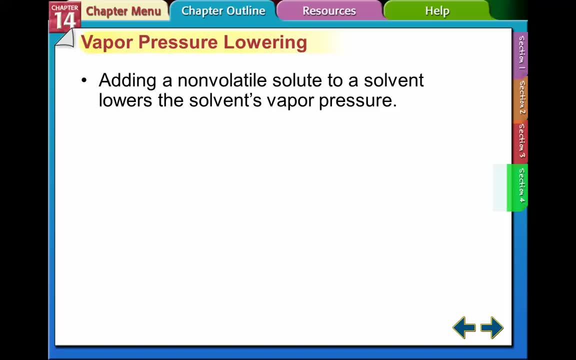 solution are strong electrolytes and many molecules do not ionize when dissolved and do not conduct electricity. Okay, so kind of a view of what ions were there. Adding a non-volatile solution to a solvent lowers the solvent's vapor pressure, So a non-volatile solute is something that's not going. 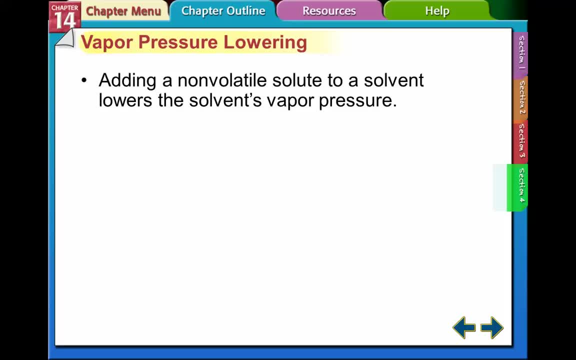 to. it's going to dissolve, but it's not going to evaporate. It doesn't have a. it's not a gas or liquid. When this solute is present- a mixture of solvent and solute- occupies the surface area. fewer particles enter the gaseous state, So it makes it harder for the particles. the gas. 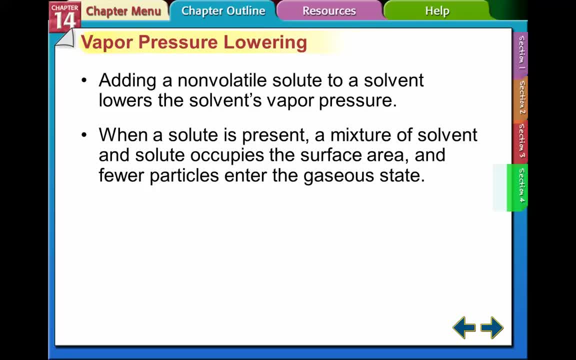 this and the solvent particles to go into the gaseous state And the greater number of these solid particles, it lowers the vapor pressure over that. Remember that boiling point was where the vapor pressure of the atmosphere equaled the vapor pressure of the liquid Well. 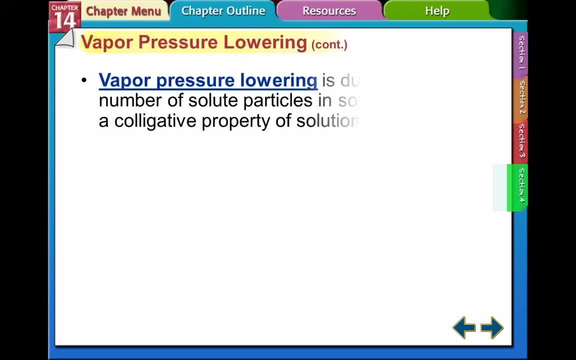 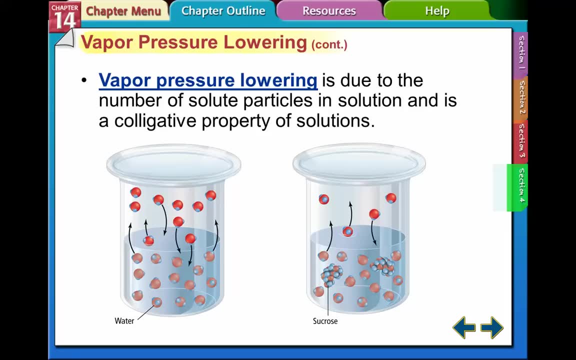 if it lowers the vapor pressure, that's going to take more kinetic energy to create that same vapor pressure we had before. So if we just have water and we dissolve sugar in it, it's going to take that more. there's going to be less water molecules above the in the vapor pressure here of 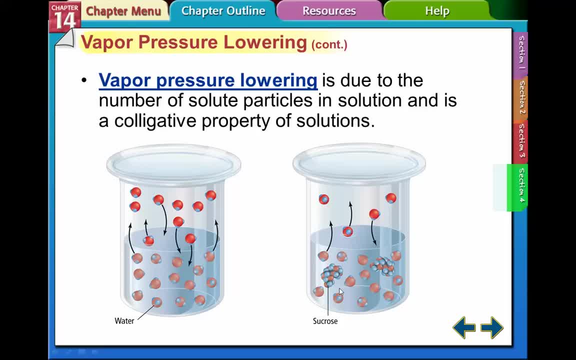 in the gas above the the water here than there would be normally. So the sugar molecules inhibit the evaporation or the. it makes the vapor pressure lower. It makes it harder for these molecules to go into solution, I mean to go into gaseous state. 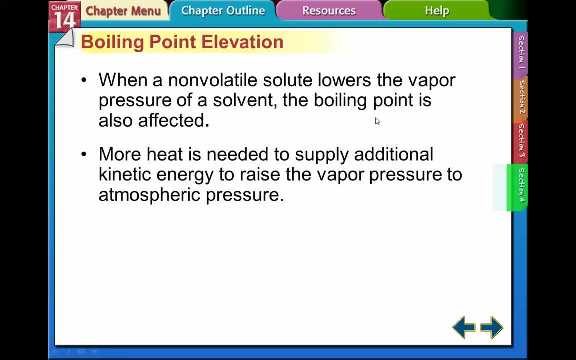 Okay, Okay. When it lowers the vapor pressure, the boiling point also is affected, because more heat is needed to apply more kinetic energy to get the vapor pressure to equal the atmospheric pressure. And that's the definition of what boiling is: when the vapor pressure and the atmospheric pressure. 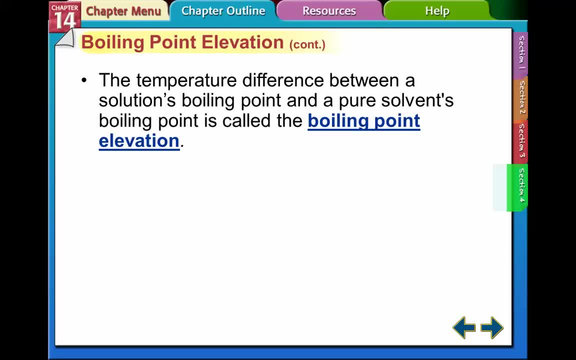 are the same. Okay, So the temperature, the difference between those, the regular boiling point and the what it's in solution, is the boiling point elevation. So stirring a solute up in the solution elevates the boiling point. You have a little mathematical formula of this, where Kb is the modal boiling. 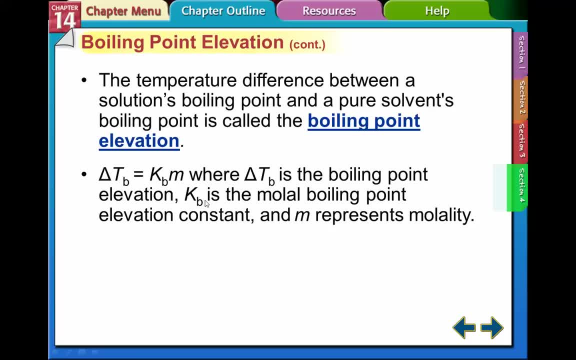 point, elevation constant, And that's the constant for whatever liquid we're dealing with here. They all the different solutions, the different solvents will have a different Kb, but the M represents the molality. right, We get the molality by dividing the moles of whatever were the solute divided by the 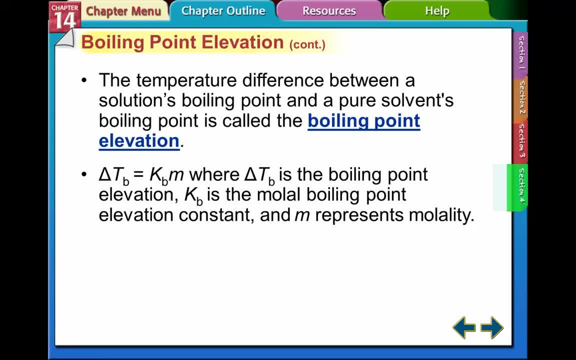 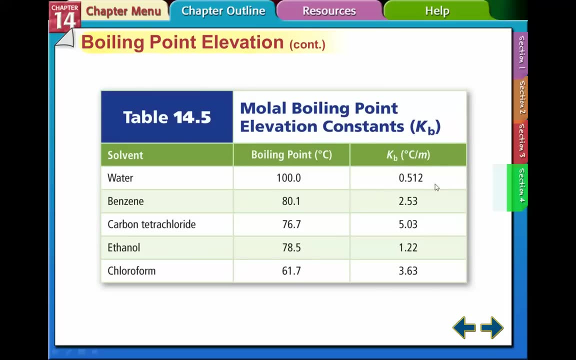 kilograms of the solvent. Okay, So that's what molality is. So it's just a pretty little simple formula And you will want to do example here in a minute. These are some of the K's, the Kb's for the boiling points, for water, ethanol. 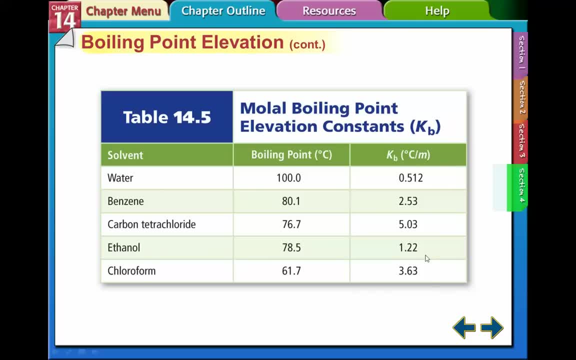 chloroform, So you'll probably have to. I forget what these are in the book, but you'll have to reference these in your book to do some of the problems you have on the WebAssign, because they talk about different things that are: 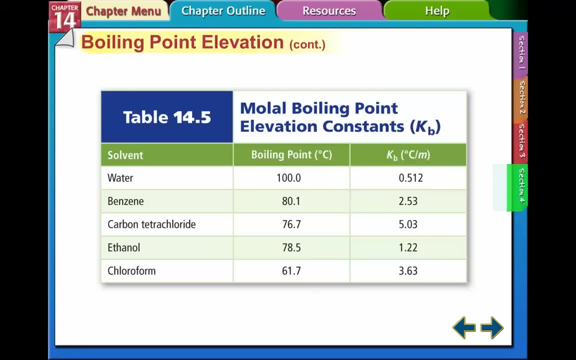 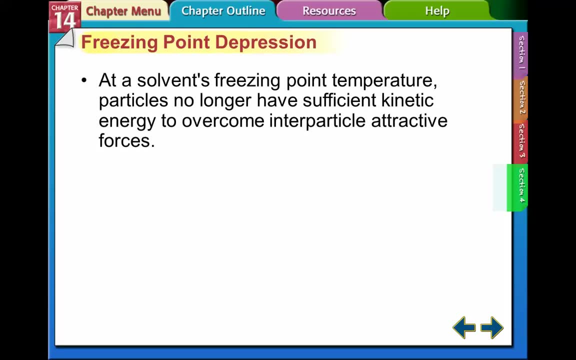 have stuff dissolved in them. what the boiling point elevation and freezing point depression. we're going to talk about that here in just a second too. so the same thing happens the other way. it says they have. when you get to the freezing point part, they want to. you know, when we have normally a freezing 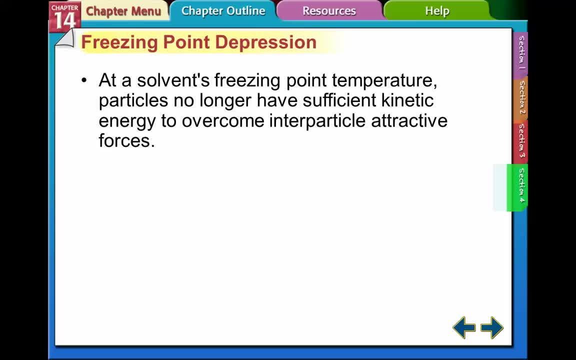 point, the inner, inner particle attractive forces. you know they come together. the kinetic energy is low enough that those inner molecular attractive forces can get together and be solid and attract each other. but if we have all this solid in there then they interfere with that and it takes 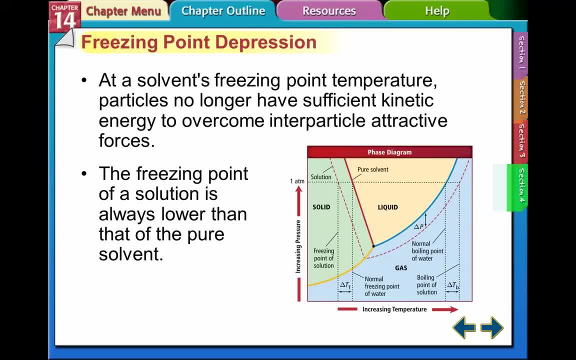 you have to have less can you have to lower the freezing points, you have to take more energy away because those solvents, the solutes I mean, interfere with that freezing process so you get a lower freezing point than a pure substance, so solid particles. if you interfere with the 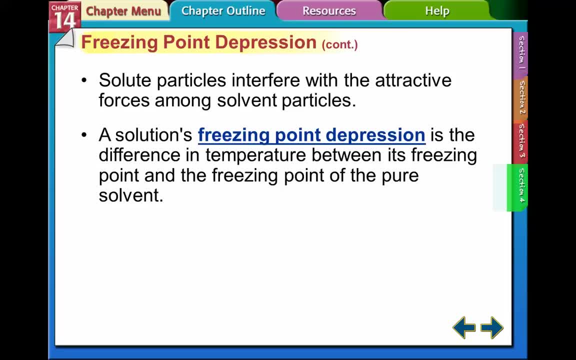 attractive voices, attractive forces among the solid, solve, solvent particles. and the freezing point depression is given by this similar, similar formula to the to the boiling point elevation. and this KF is the freezing point, depression constant. it changes forever. where they could, we really don't know. know, Mahmoud, we're dissolving in and M. 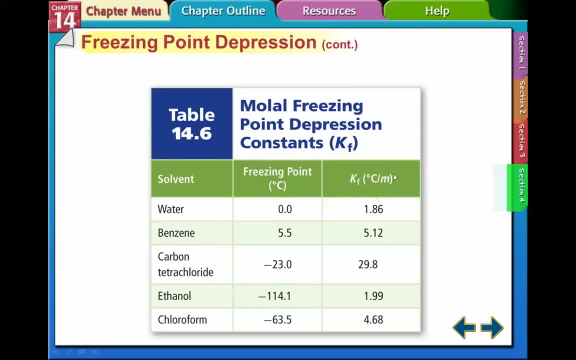 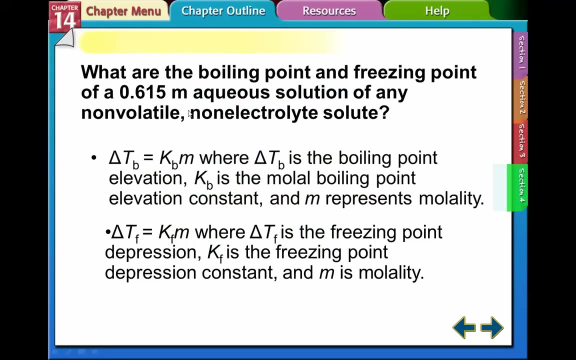 is the morality again, the moles per kilogram thing. okay, so you have a table of freezing point constance, freezing point, depression constants and this is the numbers for these different solvents. okay, so you have a question like this. this is- I got this off the Web- assign where the boiling for freezing points of 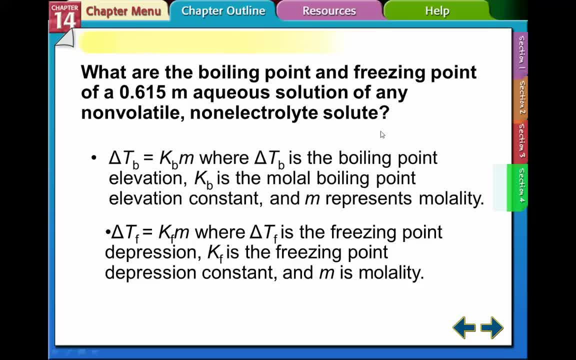 a point six, one five more: aqueous solution, non-volatile, non electrolyte solute: okay, so that's a typical solid where we can use these kb things. okay, or the kf things. so this is a review of the formulas, right, so we need to find the kb that gave. 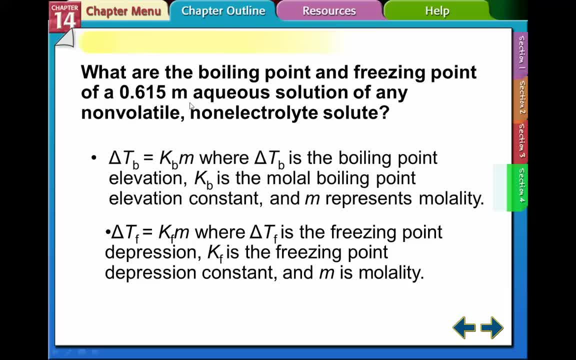 us the molarity already, the molality, i mean molality already. so we just need to figure out what this k is. we can figure out how much the boiling point went up and we can forget the k for this. well, it doesn't say what is aqueous solution, what is that? well, aqueous always means. 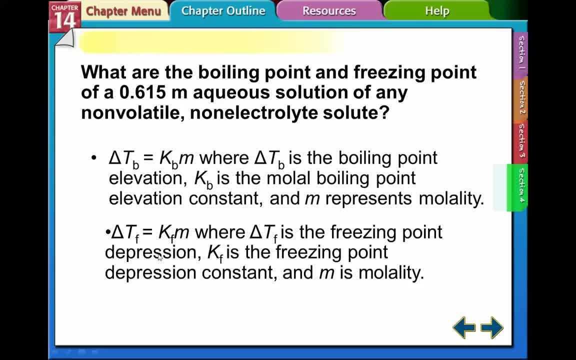 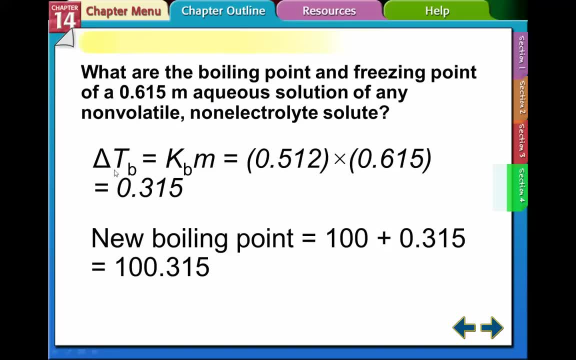 water. okay, so we just have to look up the kb for water and the kf for water. so it says aqueous solution is talking about something dissolved in water. okay, so this is the two. this is how you would get the new boiling point. this i looked up that kb for water is 0.512 multiplied by the molality. 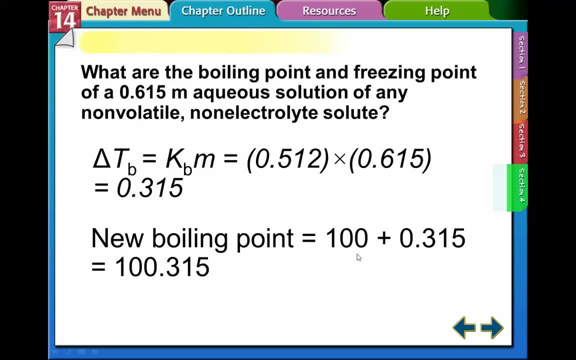 and i get 0.315. so the new boiling point is 100 plus 0.315, so it's 100.315. you have to have a whatever that you get for this difference in the new boiling point. you have to add it to what the original boiling point was. in this case. 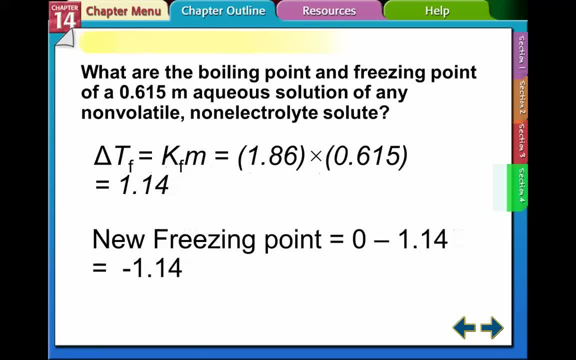 we're dealing with water, so it's 100.315 freezing point. same thing. i got the kf from the book. multiplied it by the molality, got a freezing point depression of 1.41. water freezes at zero. so when i subtract 1.14, when that my new freezing temperature- excuse me- is 1.14. so that's why. 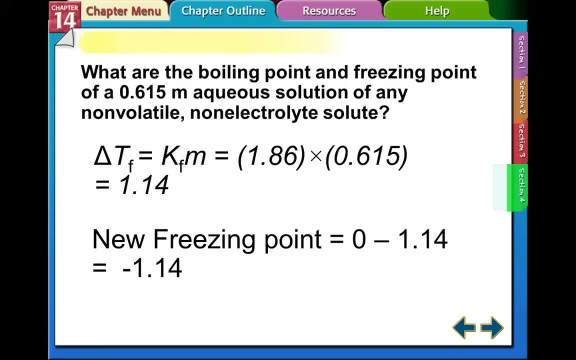 they you take. they put salt on the roads in the mountains right to lower the freezing point somewhat. so salt is dissolves in water. it creates kind of a. it makes it harder for the water to freeze. so it lowers the freezing points so the roads takes a lower temperature for the water. 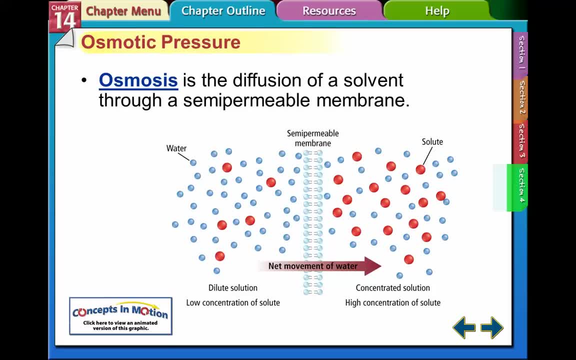 to actually freeze. you have a situation where you have a dilute solute on one side and a more concentrated one on the other side. the water is going to go to the more concentrated, it's going to go from the less concentrated to the dilute to the concentrated to kind of even this concentrations out. so that's. 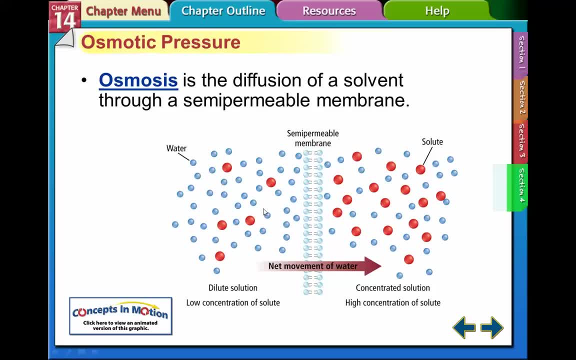 what happens when it's osmosis? it goes through and the water goes through, but the solutes stay in their respective things under reverse osmosis. you may have heard of reverse osmosis things to purify water. what they do is is the opposite: they create under pressure. they. 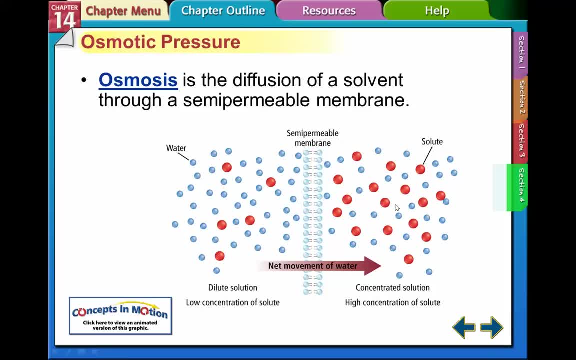 actually force these, the water molecules, to go from the concentrated side to the less concentrated side. so they leave all the solutes behind, all the salts and anything dissolved in there, and they get the pure water on the other side of that. so it creates a pure water, purified water, by leaving 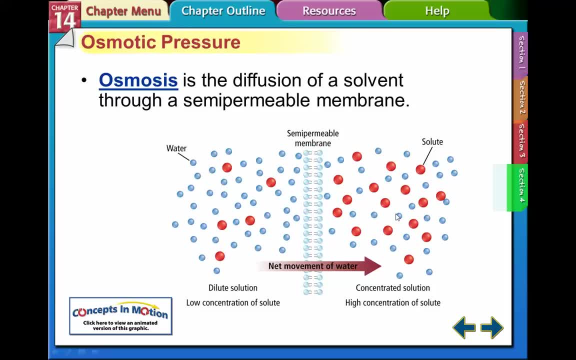 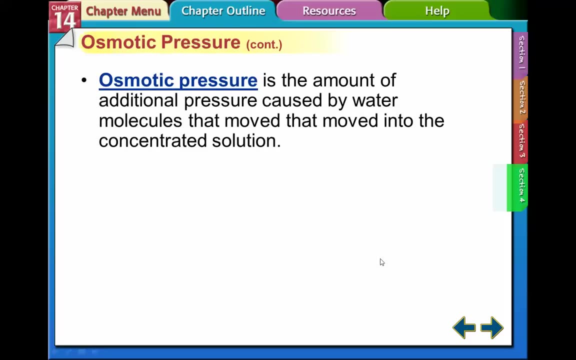 all the solutes behind. but you have to have a higher pressure on this side to force the water through and leave the solutes behind. under equal pressure situations the water would naturally diffuse from one side to the other. you go from the dilute to the concentrated side. osmotic pressure that have moved.